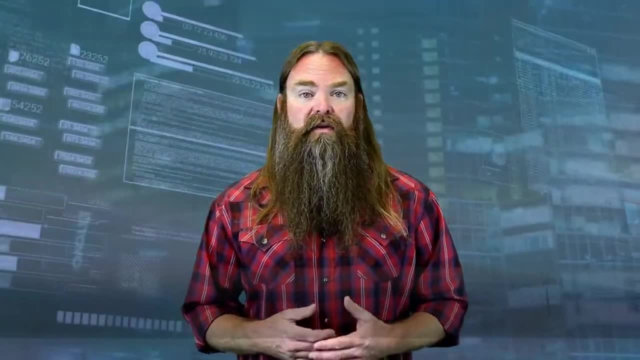 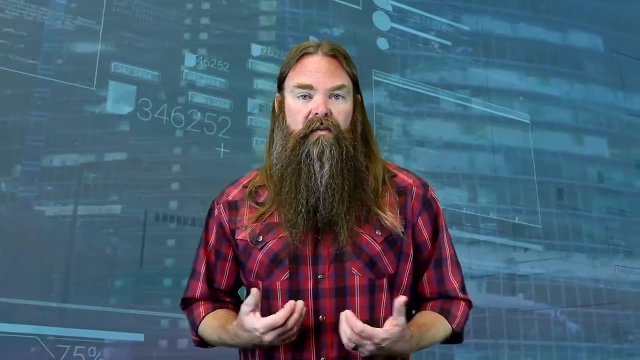 is the message we're sending back and forth: that we want to do so in a safe, secure fashion and try and guarantee that it hasn't been tampered with. we take our secret and we combine it with a key, a piece of data that is consumed by. 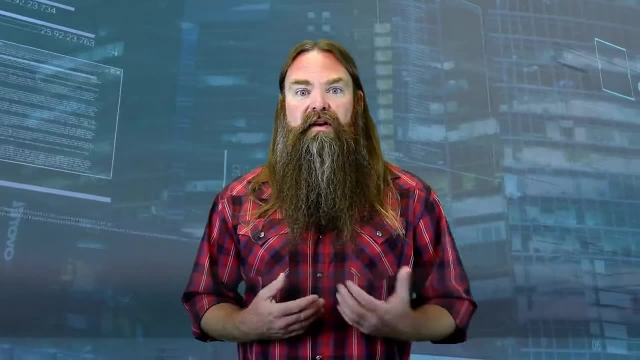 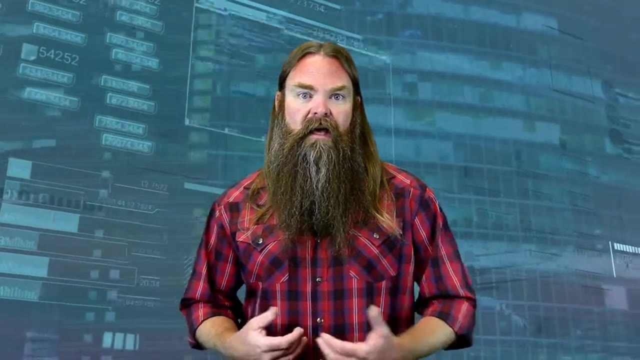 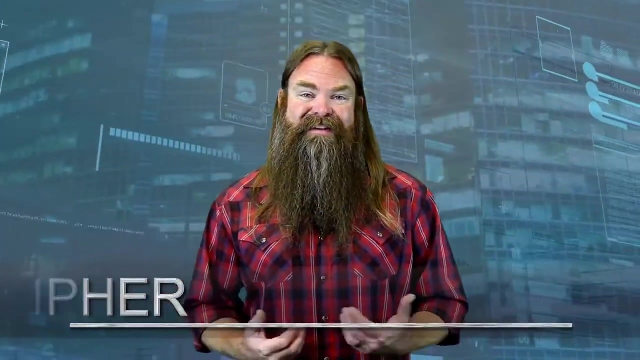 a function, our third component- when the function receives the key and the secret, the function uses the key to change the data in the secret to create the fourth and final component, which is known as the cipher. and the cipher is simply the encrypted message, the thing that, if it were intercepted, if it were seen by 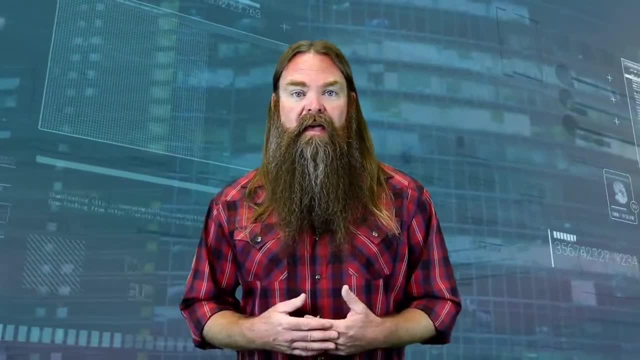 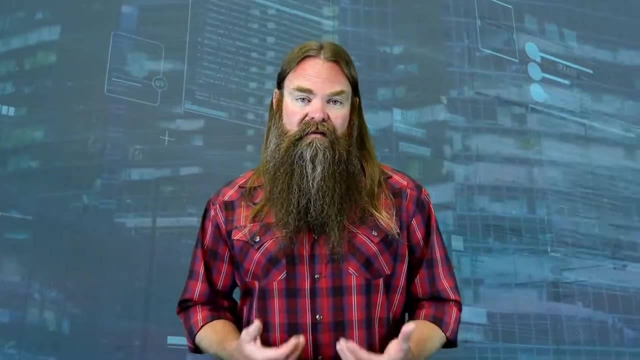 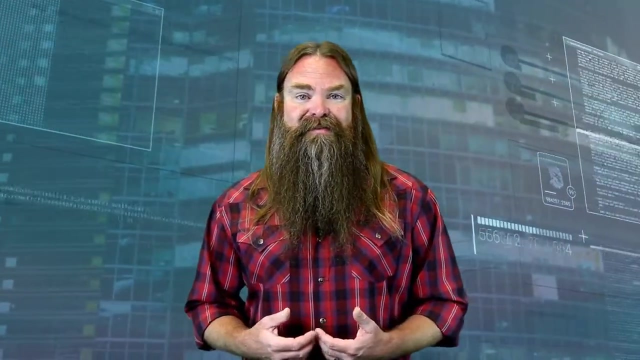 anybody else, any non participants or bad actors. they wouldn't know what the secret was, they wouldn't know what the message was and they wouldn't know how to decrypt that cipher back into the secret. now again, most cryptography functions are two-way, meaning it doesn't do me a lot of good to encrypt. 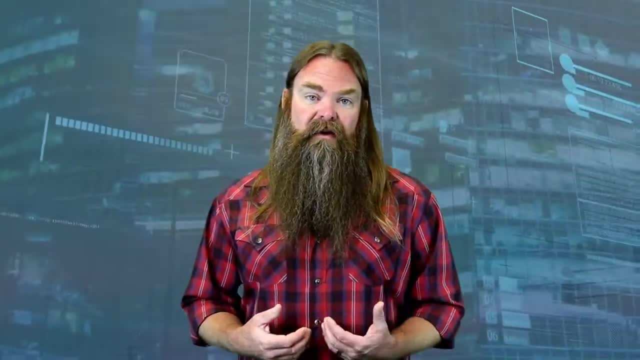 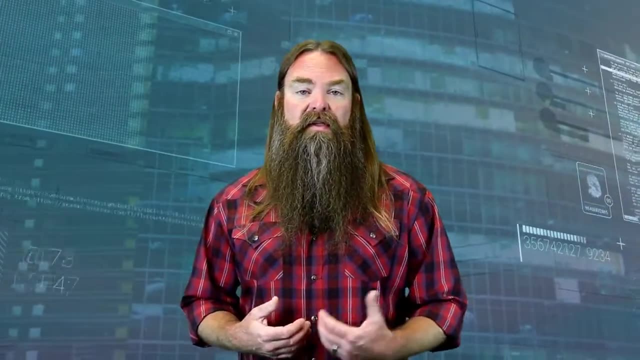 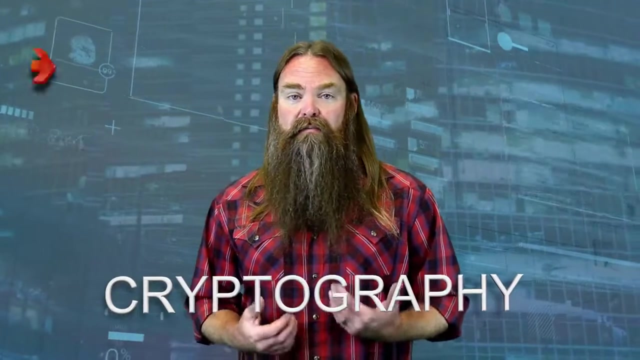 data if the receiving party at the other end can't decrypt it. and oftentimes all this involves is using the same key or reverse key into the same function, with the cipher as input to get the secret back out. so when we talk about cryptography, keep in mind those four basic components: the secret, the key, the 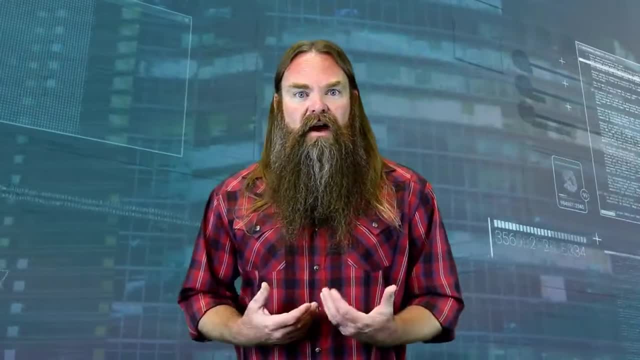 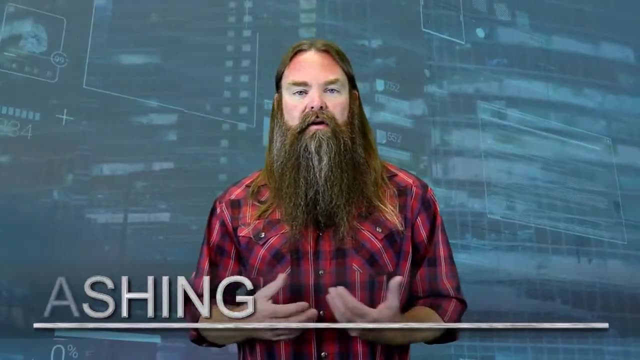 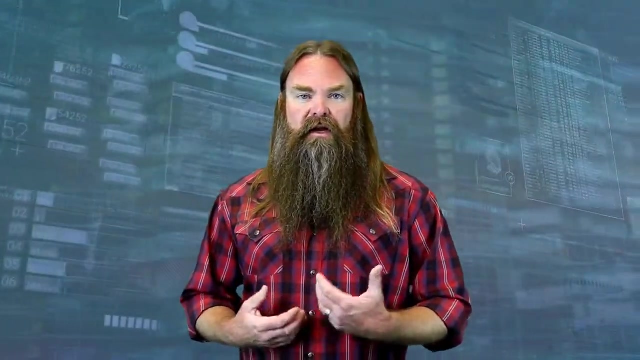 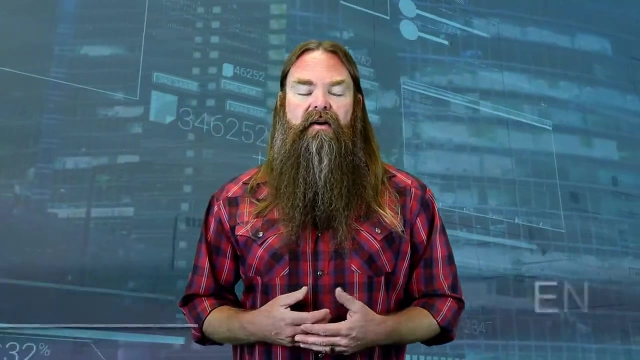 function and the cipher then understand that cryptographic hashing is a very special class of cryptographic functions which, unlike all their cousins, are only one-way, meaning that in a cryptographic hash I can put information or secret into it. the key and the function are contained as one entity and what I get back out is encoded data. I get what's called a hash. 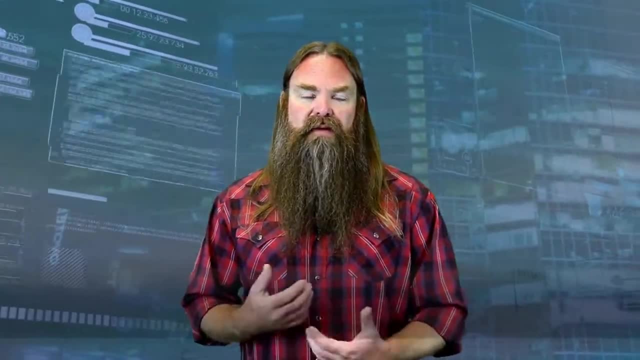 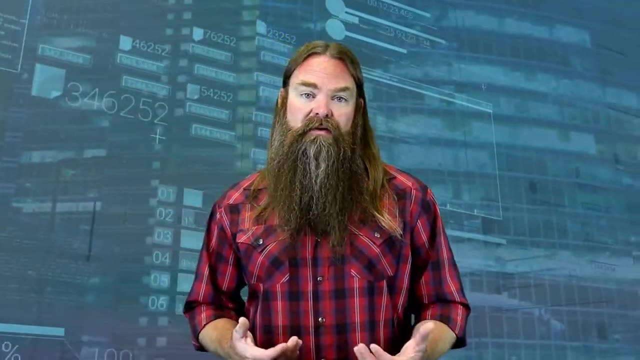 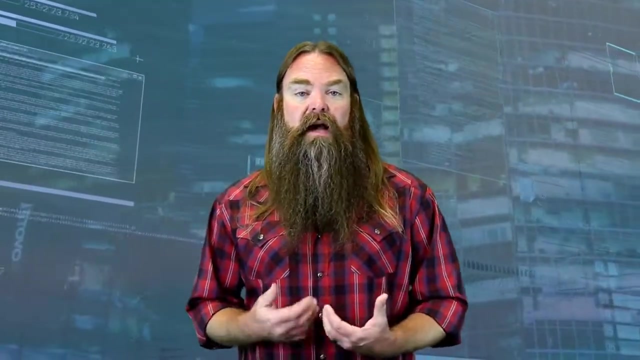 or a hash result, that is, an encryption based on the data that I put in. that is mathematically impossible to encode, reverse engineer, and this is what makes it a one-way function. if you put any data into a cryptographic hash and you share that hash with me, there's absolutely nothing i can do above and beyond random guessing, to try and recreate that input to tell me what your original secret was. cryptographic hashes are used in scenarios where we want to prove a piece of data without sharing that data, so password management systems use this all the time we don't want to store a username.